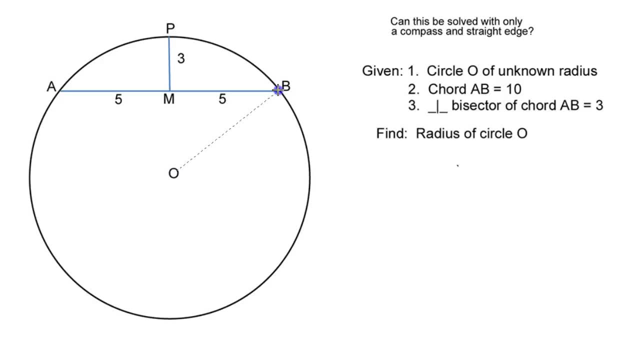 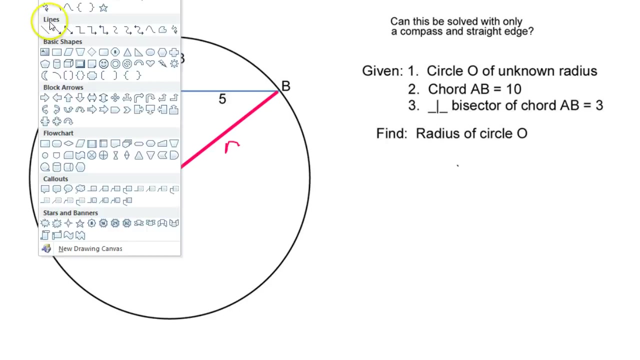 So that means we're looking for this guy right here. I think I'm going to make it pink, Alright, so we're looking for that. Let's just go ahead and call it r. Okay, now that's the radius, but we could draw another radius up in this area. 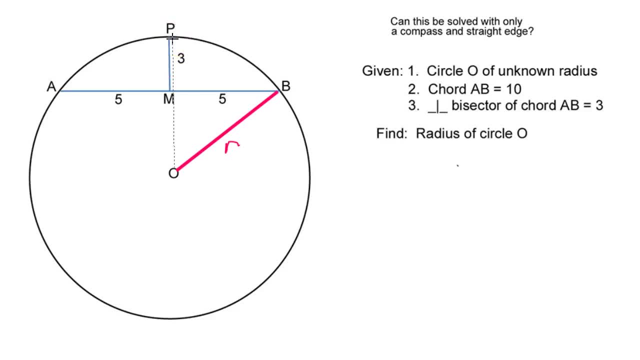 Yeah, okay, And let's see, I think I'll make this one green. Okay, so that's another radius, But, as you can see, because of the way the perpendicular bisector is, that's sort of split up into two different parts. 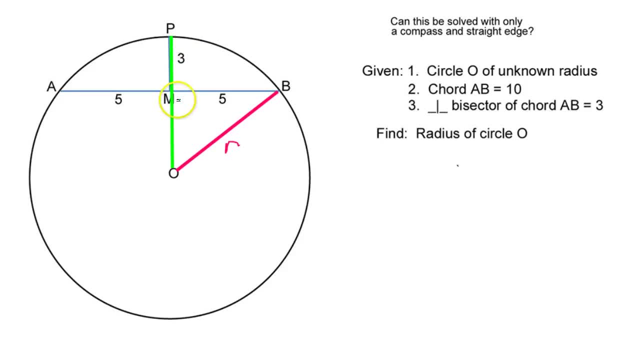 So part of it is three, So this part right here we could call it. you know, if the whole green is of course r, Just like that, Just like the pink is r, Then this portion right here will be r minus three. 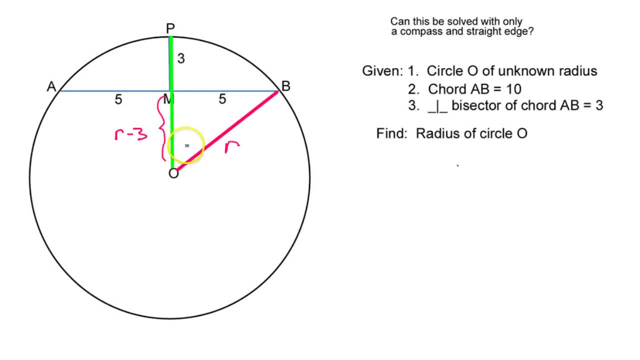 Okay, because we're taking away the three. So that leaves us with a right triangle with legs five r minus three and hypotenuse r. So you can probably guess that I'm about to do the Pythagorean Theorem. 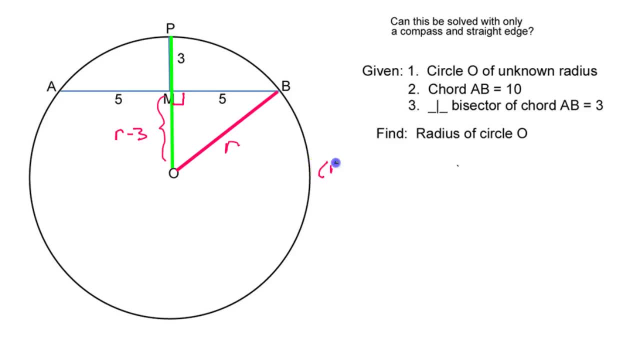 So if we do the Pythagorean Theorem, which would be r minus three squared plus five squared is equal to the radius squared. r minus three squared is r minus three times r minus three. Okay, of course. five squared is 25, is equal to r squared. 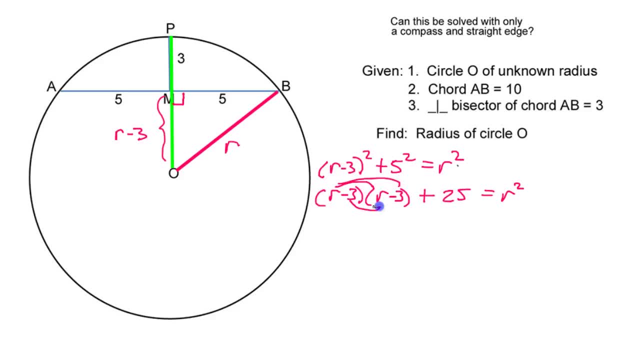 Alright, if we FOIL this or use the double distributed property, whichever way you like to look at it, we are going to get r squared minus three, r minus three, r plus nine from that, And then we're bringing down the plus 25, is equal to r squared. 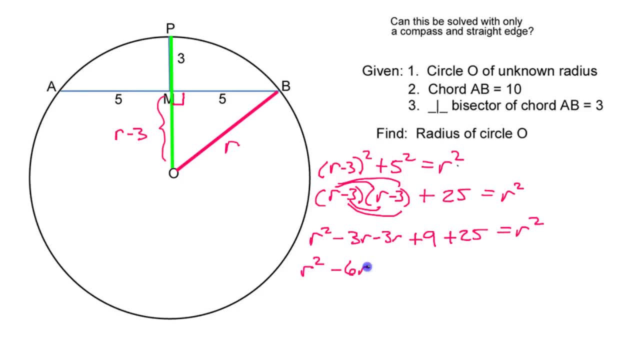 So that's going to be r squared minus six r plus okay, putting these together, that's going to be thirty-four equals r squared. Now I'm going to go ahead and write this down. Notice, we have r squared on both sides.